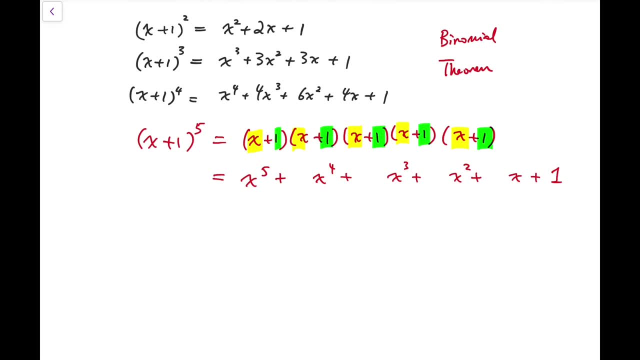 Say how many x to the power 5 are there, How many x to the power 4 are there, et cetera. For x to the power 5, we need to choose x from all. 5 copies of x plus 1, underlined in black. 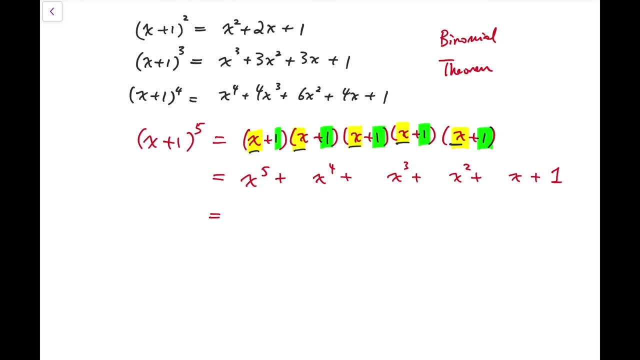 So that means that We need to choose all 5 objects among 5,, which means there are so-called 5-choose-5 number of ways to get x to the power of 5.. And similarly, for x to the power of 4, there should be so-called 5-choose-4 number of ways. 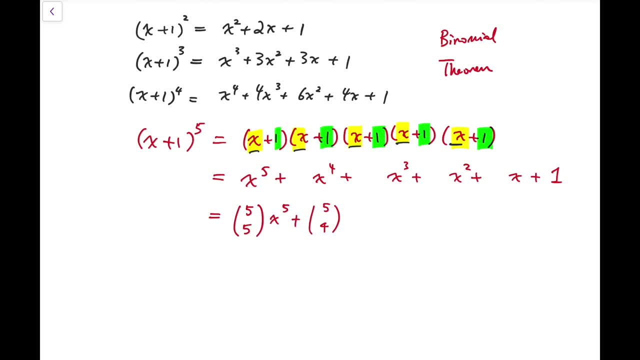 to choose 4x among the 5 copies of x plus 1, and then the rest, and for the remaining 1,, 1 will be choosed, and so the outcome will be x to the power of 4.. So, using a similar argument, we'll have the expansion to be these two terms added by 5-choose-3. 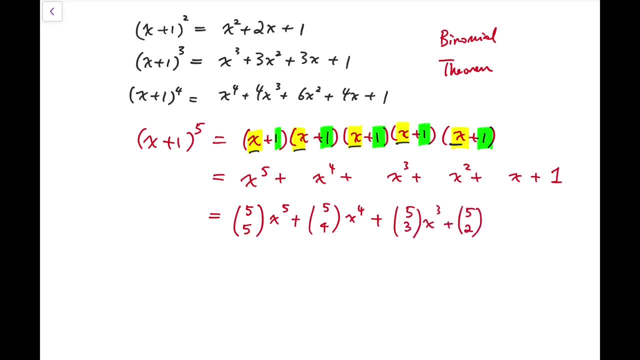 times x cubed, plus 5-choose-2 times x squared, plus 5-choose-1 times x plus 5-choose-0 times 1, and it's just 5-choose-0 itself. Okay. 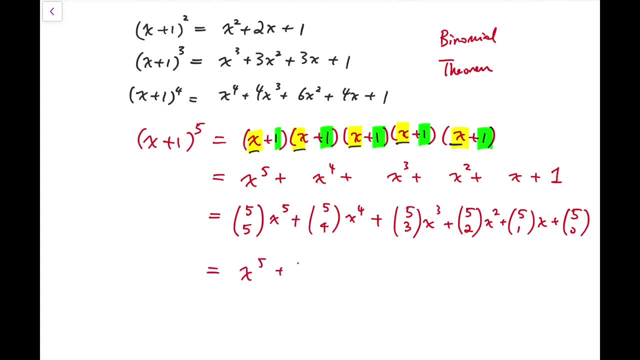 And it turns out to be x to the power of 5 plus 5x to the power of 4 plus 10x to the power of 3 plus 10x squared plus 5x plus 1.. But in this problem it's not important on how do we compute each of the binomial coefficients? 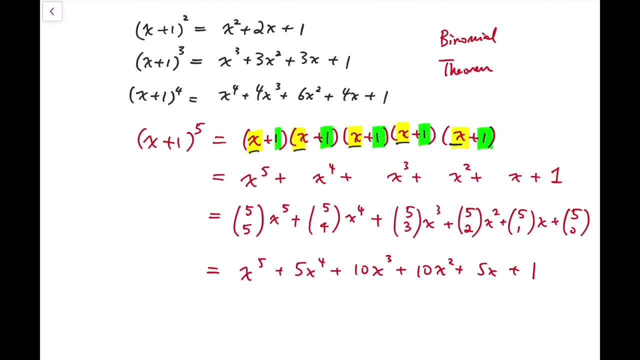 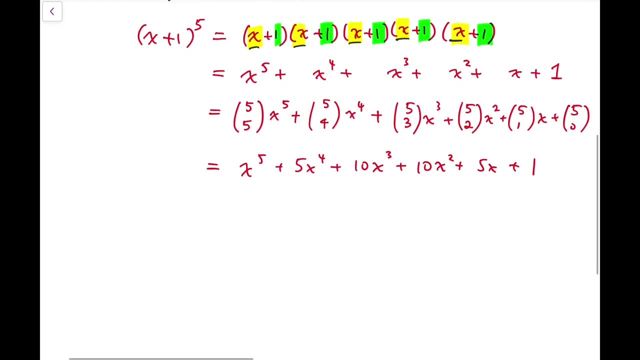 so we'll just skip that. The series is just for your information. Now, using what we've got, we can deduce that, Okay, The expansion of x plus 1 all to the power of 20 will be something like 20-choose-20 times. 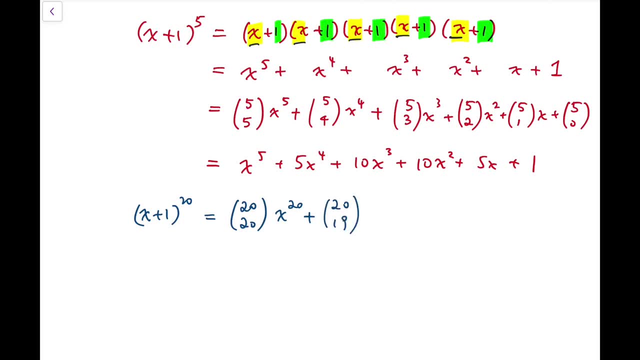 x to the power of 20, plus 20-choose-19 times x to the power of 19,, 20-choose-18 times x to the power of 18, adding all the way down to 20-choose-2 x squared plus 20-choose-1 times. 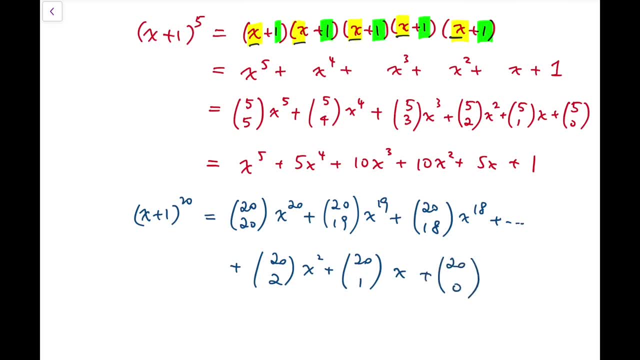 x plus 20-choose-0 times 1,, which is that number itself, And you may notice that we have the coefficients to be exactly the numbers that we want to add Now at this point. here is the key trick: If we replace all the x by 1.. 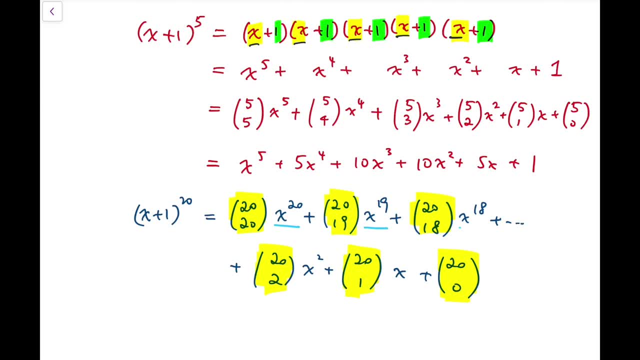 So that, Okay, So these terms, the underlying terms, will all be omitted, because the number multiplied one is just a number itself. And of course we can do that because what I've written just now is actually an identity, which means this should hold for all values of x. 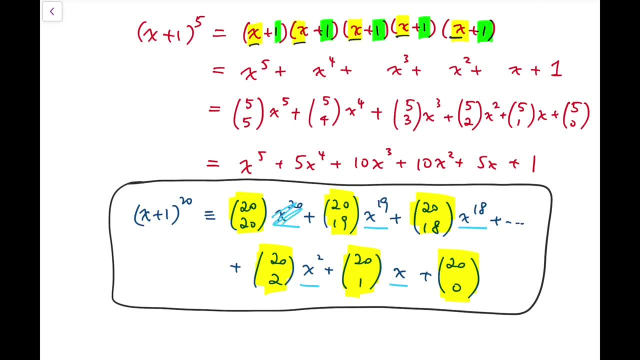 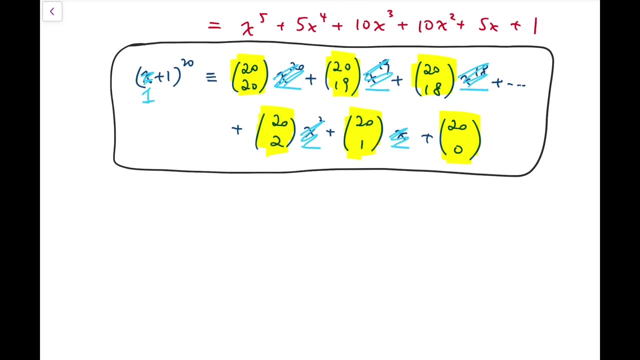 So, in particular, I can replace this: Okay, So this is x by 1. And so these numbers can be ignored, and we have the sum of the coefficients, And this number turns out to be 1 plus 1, all to the power of 20.. 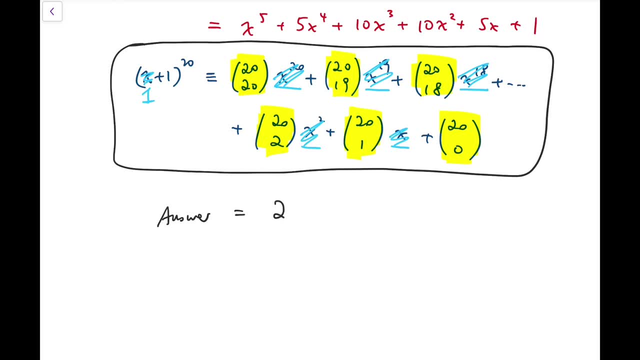 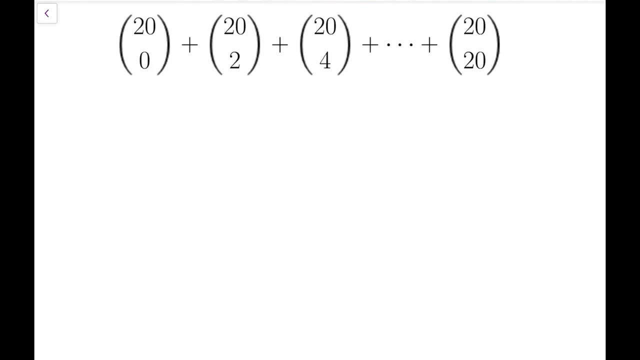 So that means our final answer should be 2 to the power of 20, and that is equal to 1,048,576.. So this is the answer to our problem. Okay, I'm going to end this video by evaluating this sum as some sort of extension of what? 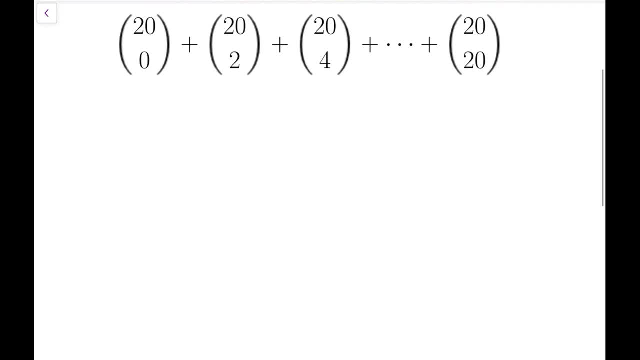 I've done previously. As you can see, the numbers 20 choose some odd number, say 20 choose 1,, 20 choose 3, and so on, are omitted, And to evaluate this we need to consider multiple binomial expansions. 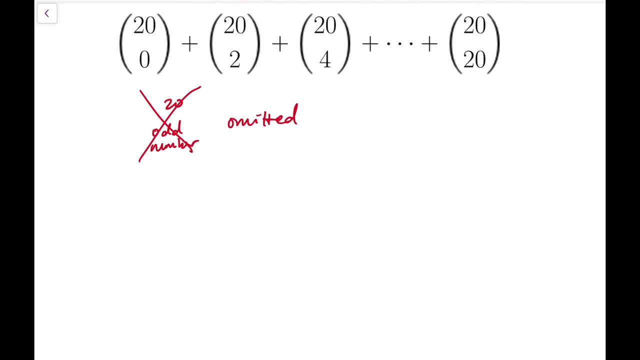 Okay, Notice that if we add all the terms of the form 20, choose r, where we have no restriction on r, just between 0 and 20, then we will have the sum to be equal to 2 to the power 20.. 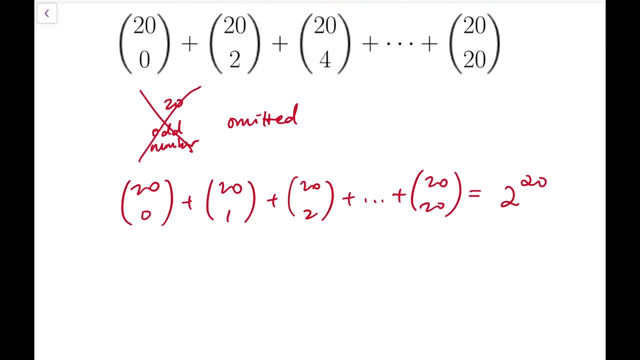 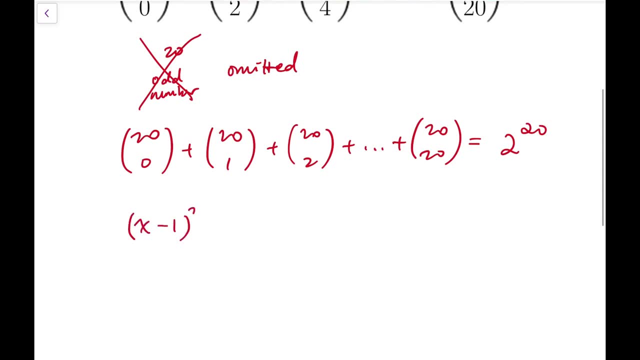 So we need to subtract out the terms of the form. 20 choose odd number. Okay, To do this, let's consider the expansion of x minus 1 all to the power of 20 instead, And it turns out it's exactly turning the coefficients of odd powers to negative, while 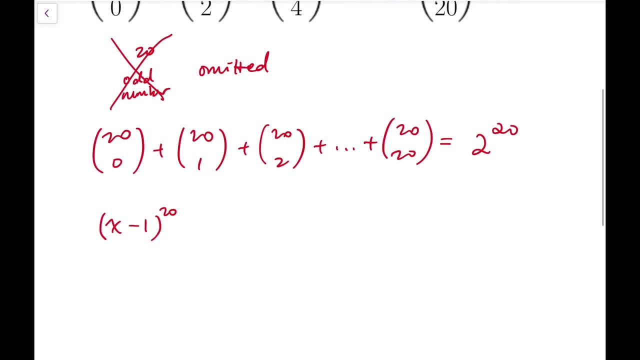 the coefficients of even powers remain the same, So that means it should equal to 20. choose 20 times x to the power of 20. minus, not plus, but minus 20.. Okay, So this is the result: Not plus, but minus 20. choose 19 times x to the power of 19,. plus, because it's even. 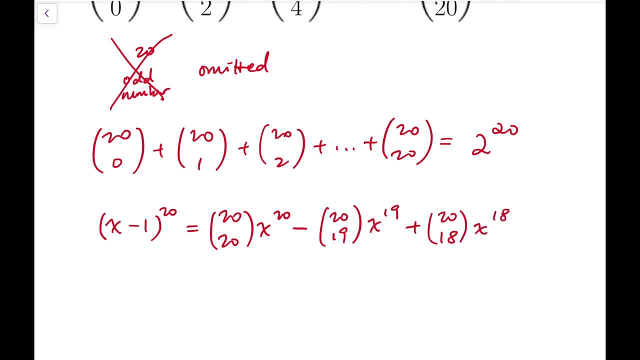 powers: 20. choose 18 times x to the power of 18, and then minus again 20. choose 17 x to the power of 17,, and so on, And then last we'll have minus 20. choose 1 x plus 1 again, because constant term means. 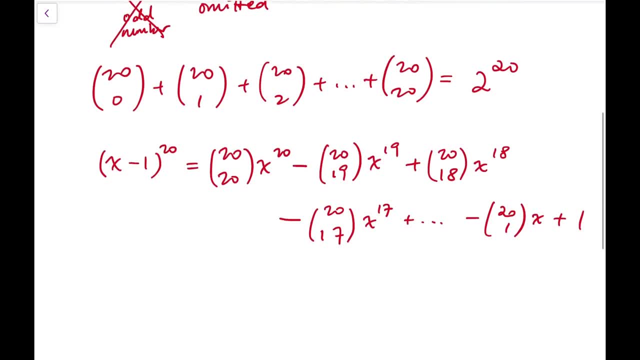 0 power, And that's even Now for this expansion, if we replace x by 1 again. so that means I'm removing all the x terms like before. And then this sum: adding all the 20: choose even numbers. subtracting all the 20: choose. 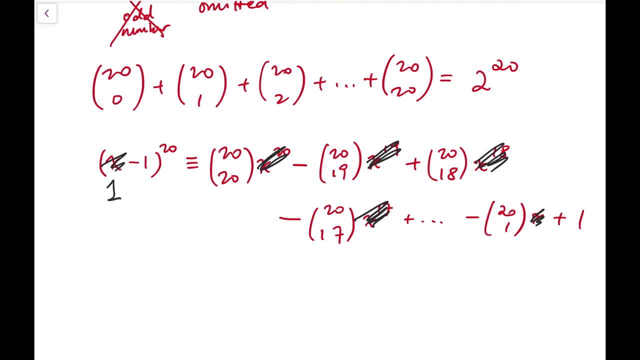 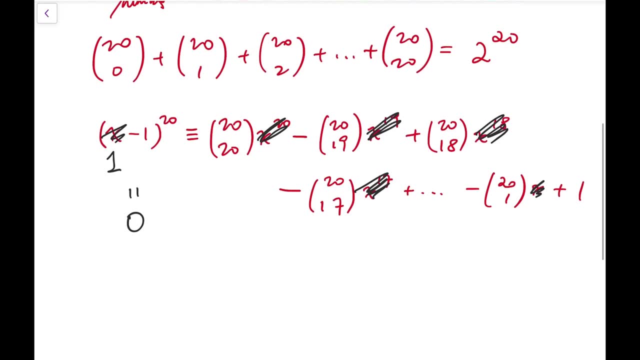 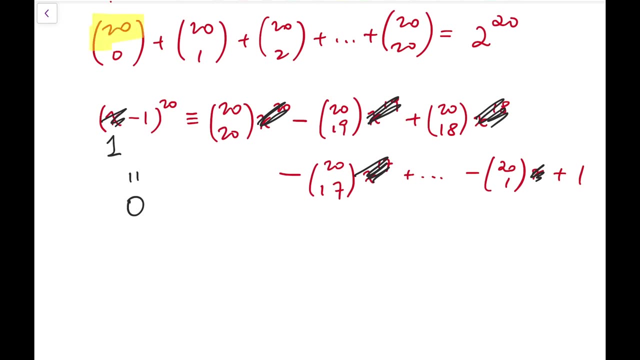 odd numbers is actually equal to 1 minus 1, all to the power 19.. Okay, So that's equal to 20, and that's equal to 0.. Now, to evaluate the sum we want, we can actually add the two results. we've got this one. 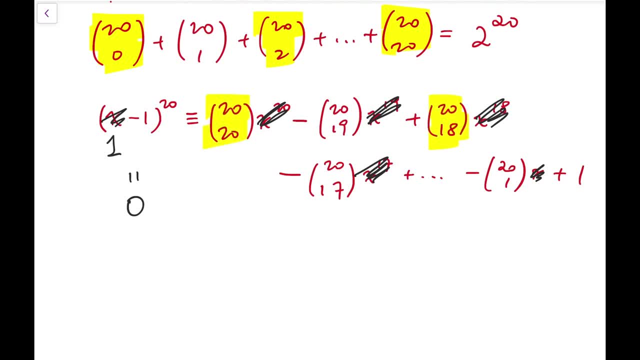 We add in these terms, while subtracting or I should say canceling out all the terms of the form: 20- choose odd numbers, While we have two copies of 20, the sum of 20- choose even numbers. So 2 times our final answer equals 0 plus 2 to the power 20..